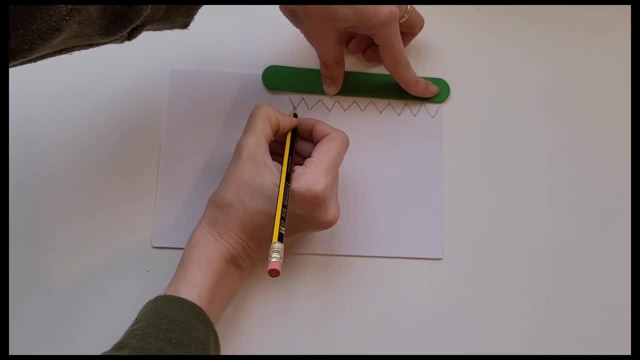 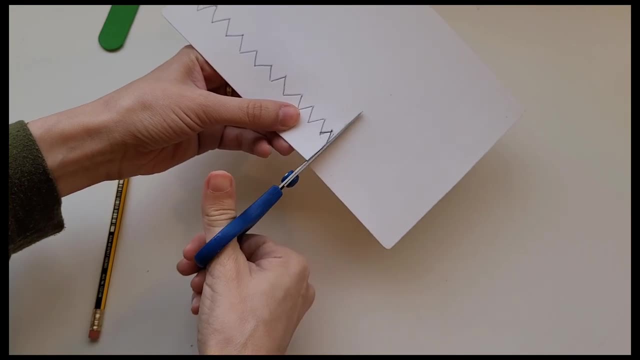 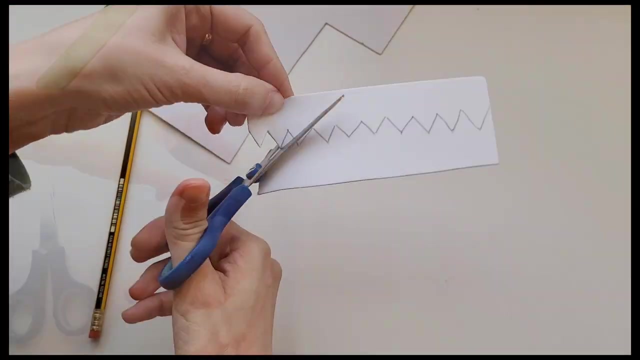 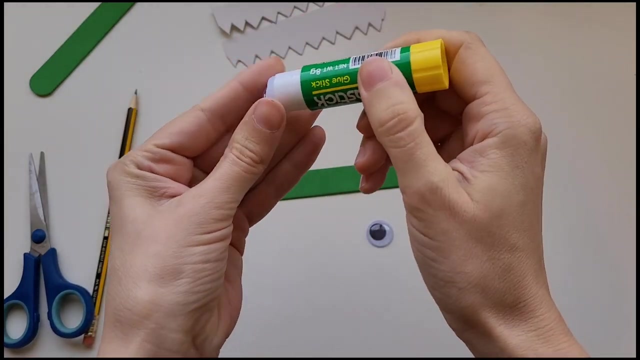 We're going to use green craft sticks and then we're going to trace out some teeth on the white foam. After we trace out the teeth, we're going to cut them out. Music: Then we're going to get some googly eyes and we're going to stick them. 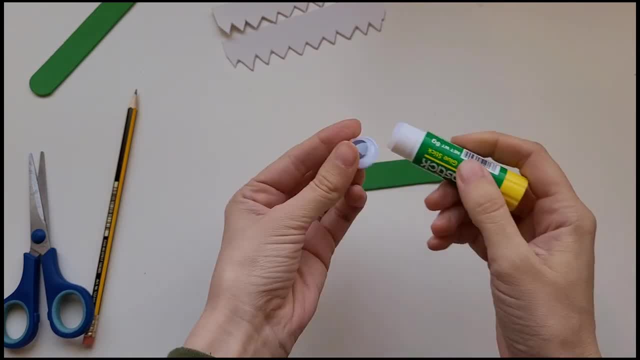 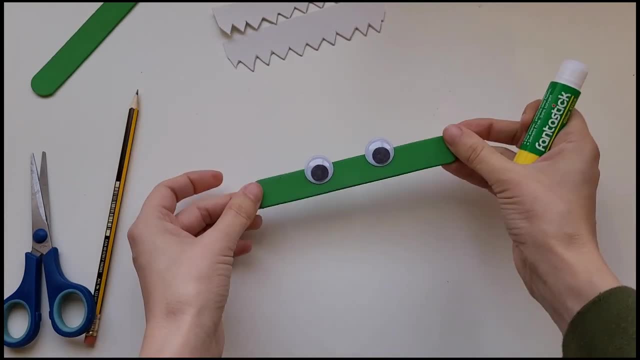 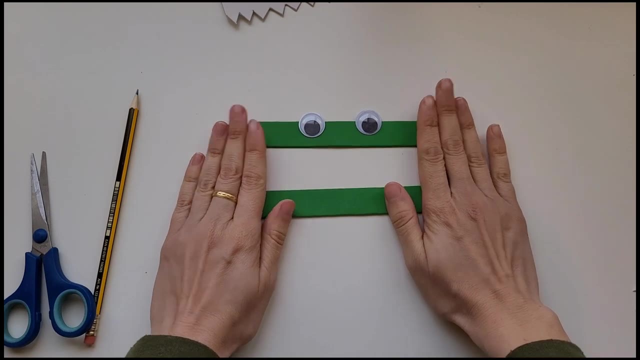 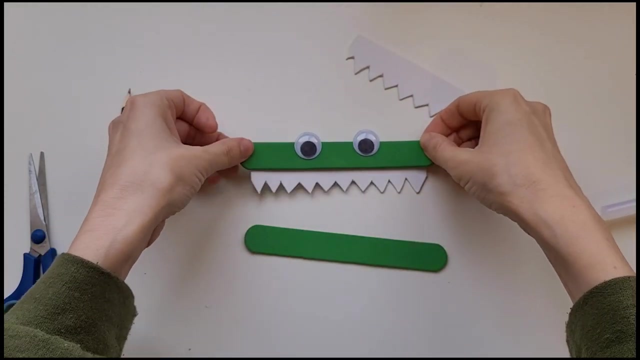 on the top part of one of the craft sticks: Music, Music. Now we're going to use a glue gun to fasten the teeth onto the craft sticks. We're going to fasten them on the back side so that the glue doesn't show. 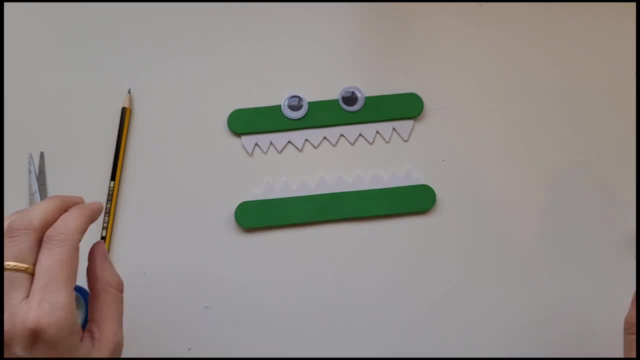 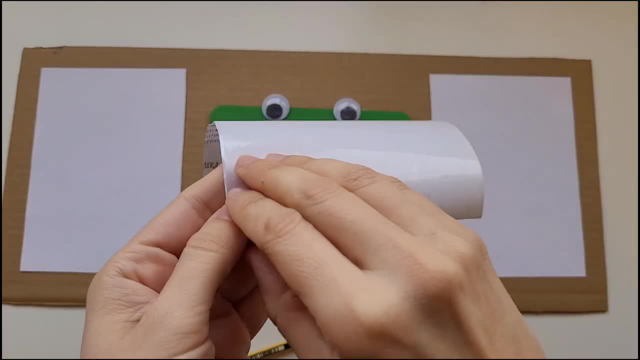 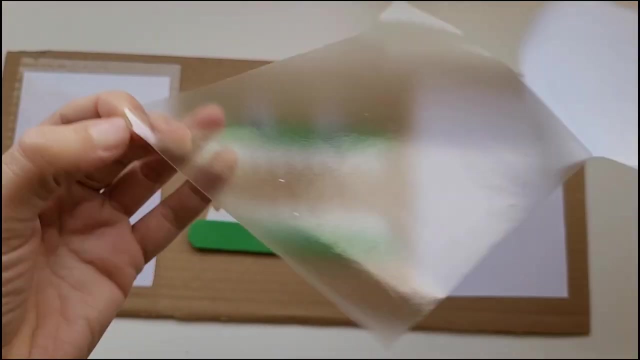 After we've fastened both sets of teeth, we can now move on to the next step. We are going to take a piece of cardboard and we're going to put two pieces of white paper on either side. Then we're going to cover the white paper with clear lamination. You can also use 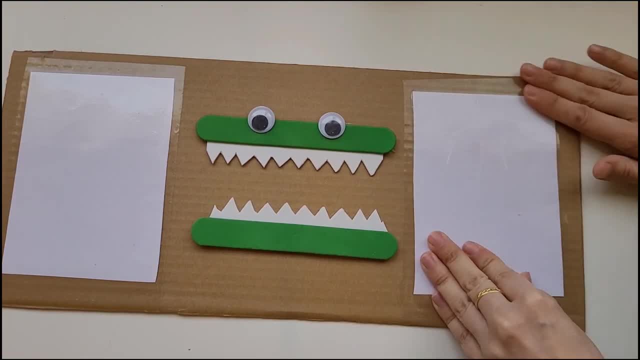 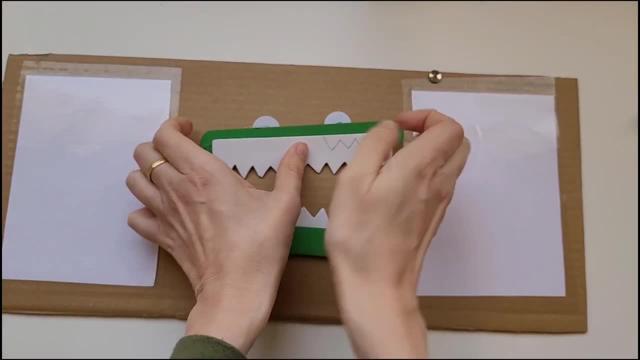 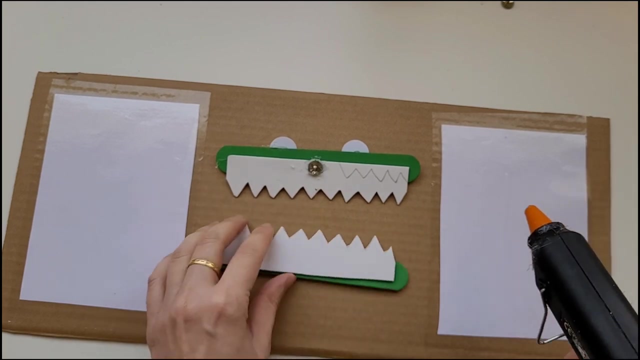 clear tape for this step: Music. Next, we're going to use these tacks or push pins. We're going to glue them on the back side of the craft stick. We're going to make sure that they are in the center. After we glue the push pins on the back side of each craft stick, we can now turn them over. 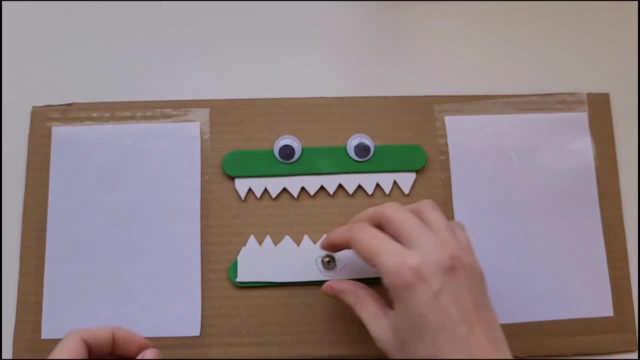 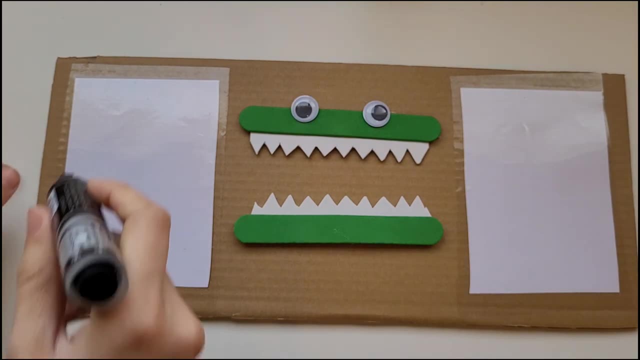 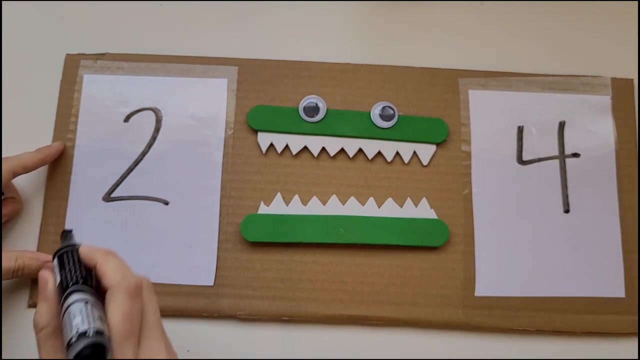 and place them into the cardboard. If your cardboard is not thick enough, you can put two pieces of cardboard on top of each other and just glue them together. Now we have an alligator. Using a dry erase marker, we can write a number on each square. 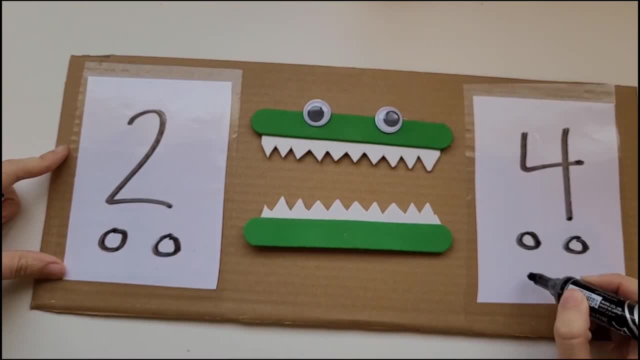 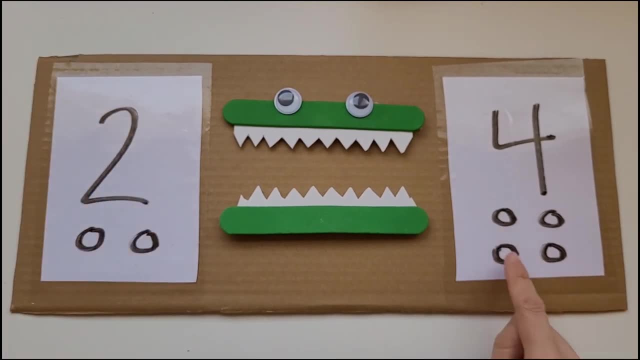 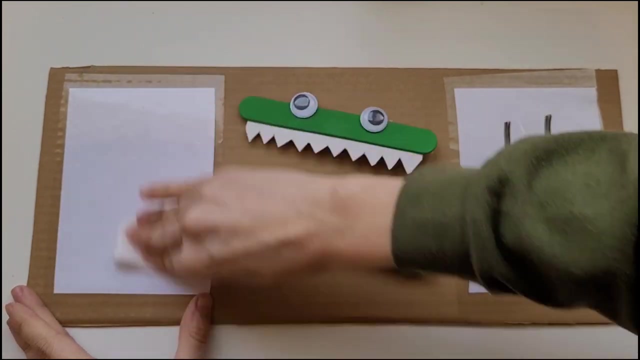 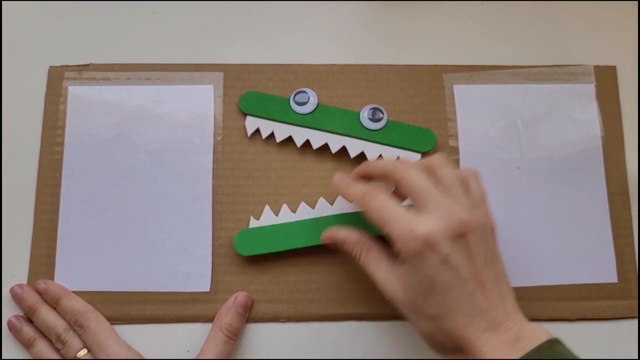 We can also draw circles to show what each number represents. Then your child can compare the numbers by either looking at the numbers or counting the circles, And then they will use the alligator to make the greater number. After you're done, you can erase this and use it multiple times.